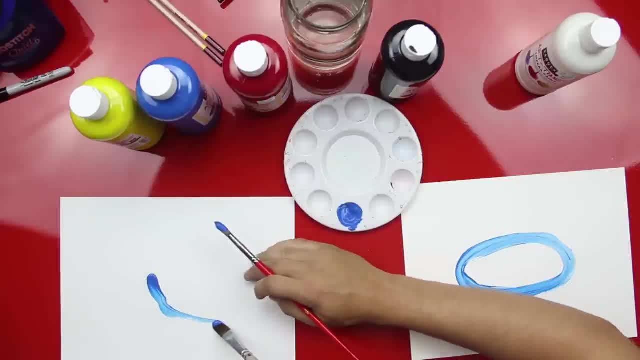 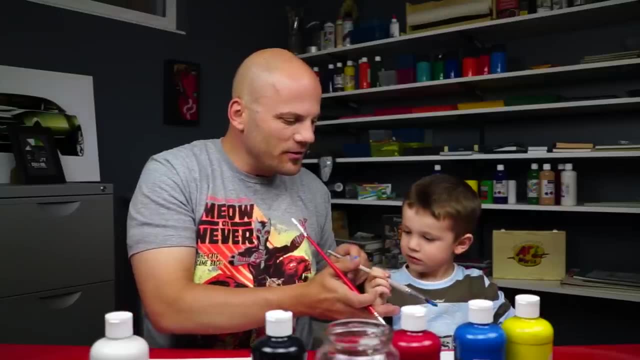 oval. Yeah, Okay, do a big oval. Hold your. hold your uh paper with your. oh, you got me. Okay, hold it like a pencil. Hold your hand down a little further. I got you. Yeah, you got paint on my finger. Look at that, I'll wipe it. 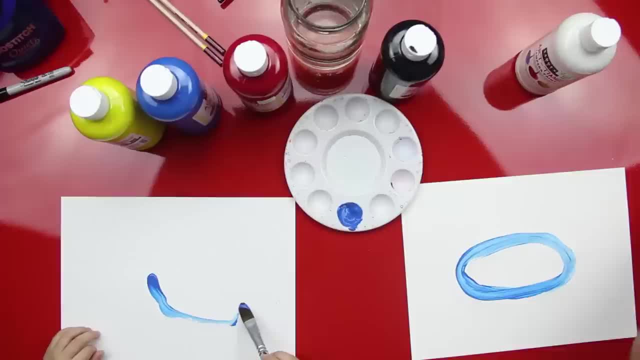 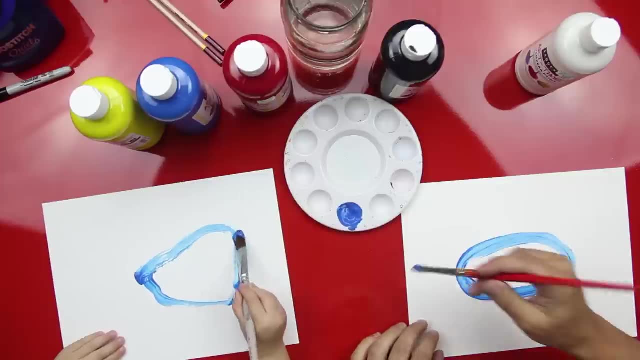 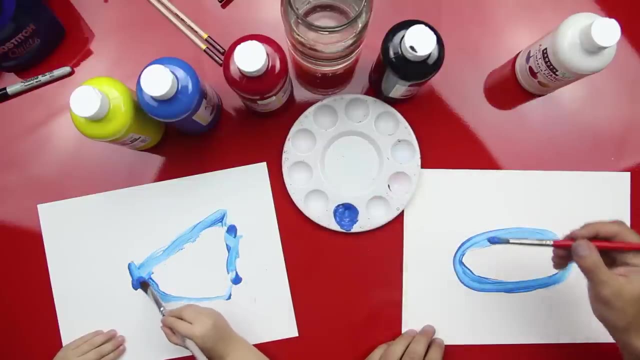 off, It's okay. All right, make your oval really big. Hold your paper. Good job, That's. that's perfect. I can make it. Yeah, get some more. You're running out. Okay, now, get some more and we're gonna color it in. Paint your oval, Paint inside your oval. Okay, Get more. 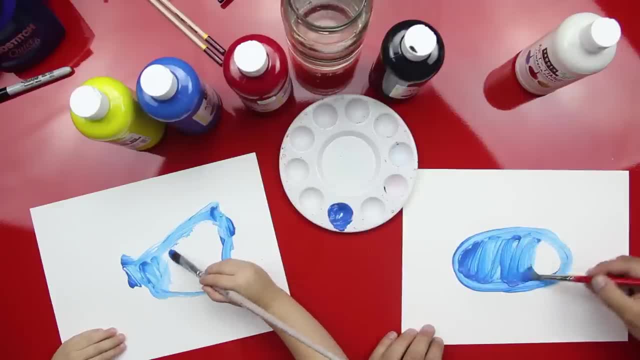 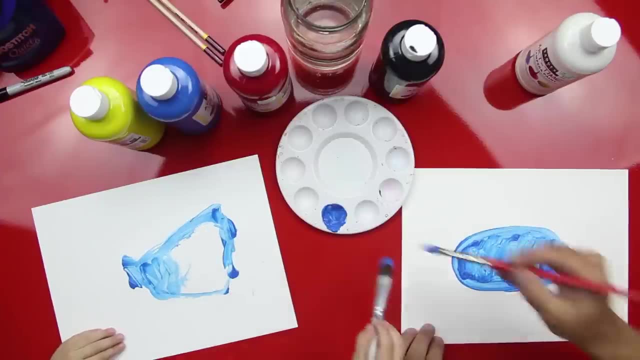 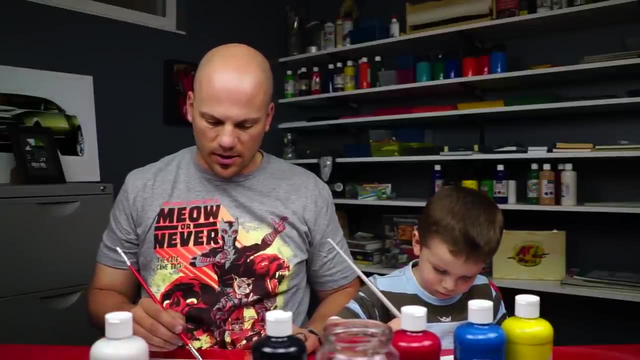 blue. if you run out. Do you like painting, Austin? Yeah, Yes, I like painting with you. I run out. Okay, get more. Paint the inside. This is a good. this is a good, uh, art activity with your young. 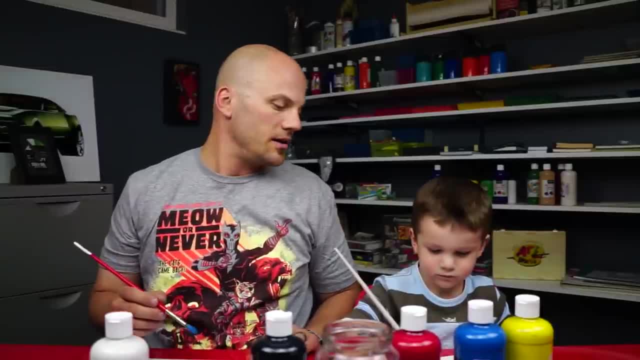 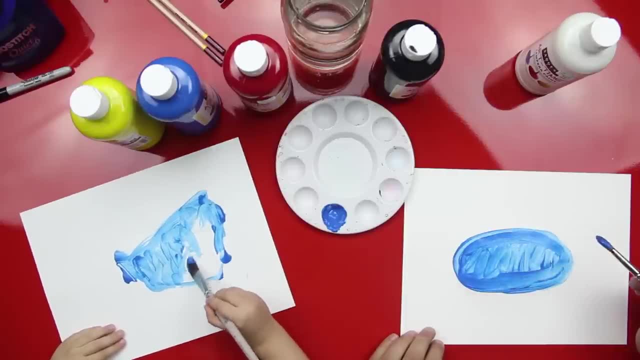 artists. Do you talk about shapes? Yeah, You can talk about shapes. Yeah, You can talk about colors, and you can talk about drawing the shape or painting the shape first and then painting inside of it. so it helps them learn control. Keep going. You need a little more, That's okay. 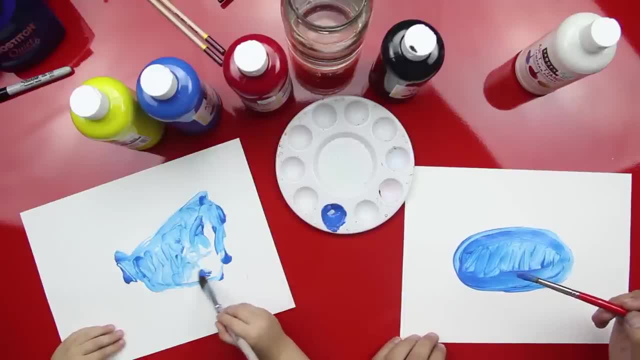 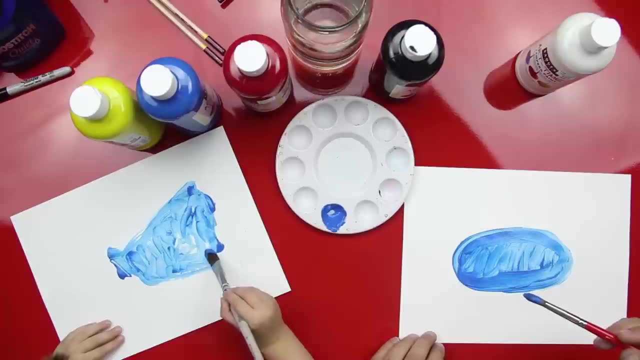 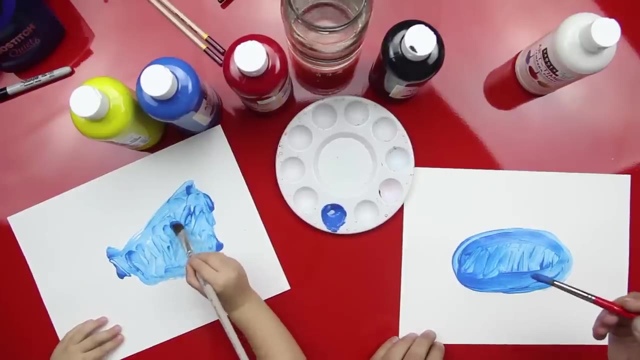 Keep going. We want, we'll wipe it up, clean it. With just a little bit of instruction, you can see it gets really focused and concentrates. huh, You're concentrating. Yeah, Yeah, Good job, Austin, You did it. Okay, now I'm gonna square it a little more blue. 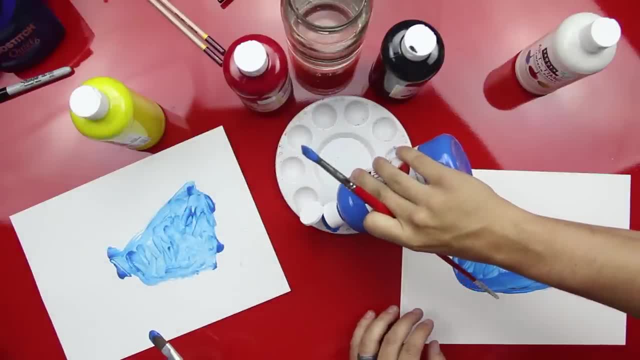 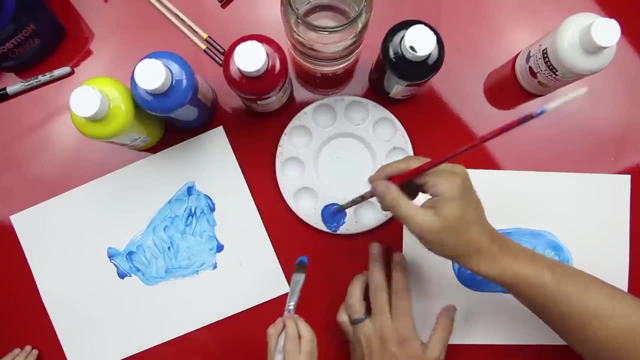 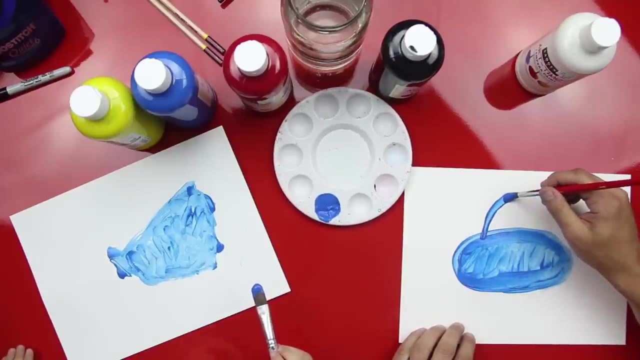 and we're gonna paint the top of the car. Okay, Okay, And we're gonna use a rainbow line to paint the top of the car. Okay, you get a little more blue and watch this. Watch, dad. We're gonna do a rainbow line that goes up and down. Can you do that? Yeah, Up and down. 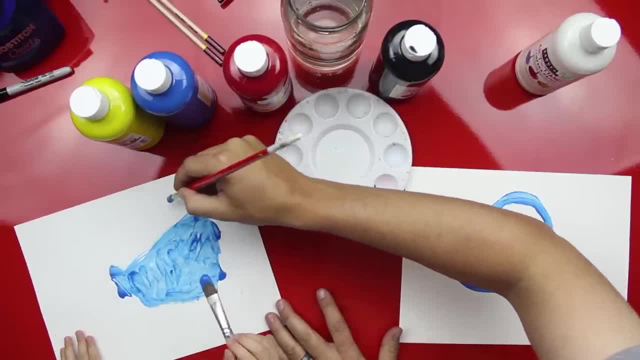 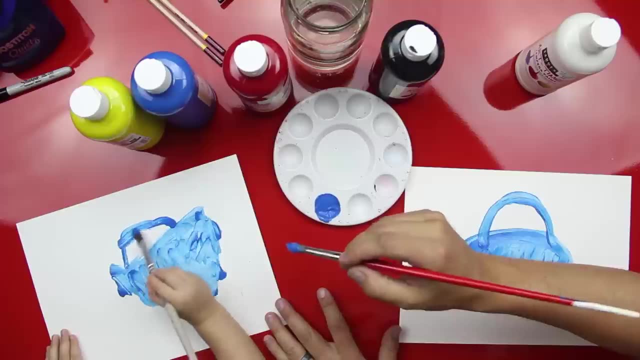 Let's do it. Start up here. Mm-hmm, Start up here, Go up and then down. Yes, You did it. Look at that. Okay, don't color it in yet. Okay, now we're gonna do. 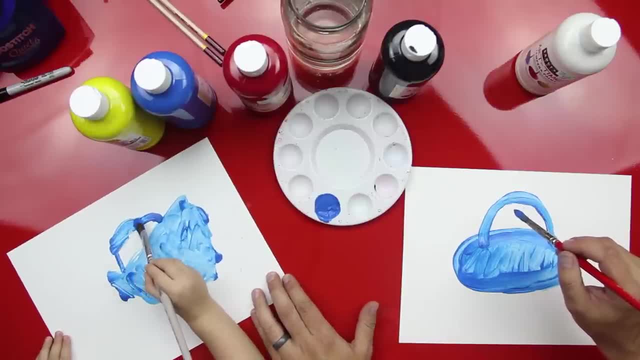 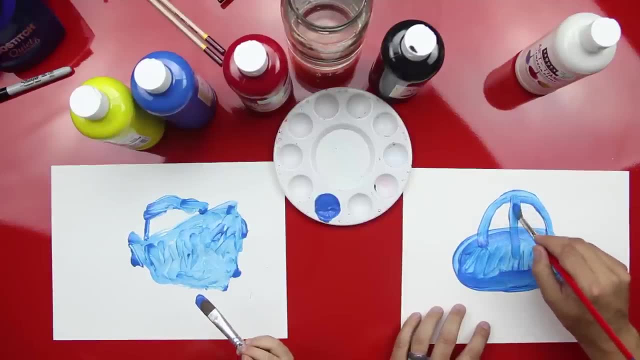 a line, Got it? Yeah, Good, Okay, watch this. We're gonna do a line right down the middle. Can you do a line down the middle? Yeah, Right in the middle. Good, And that's it, And you're done. 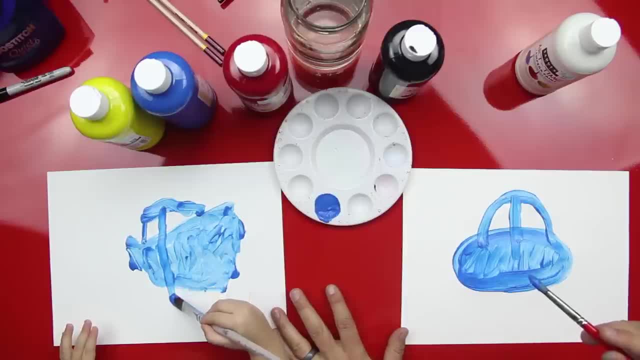 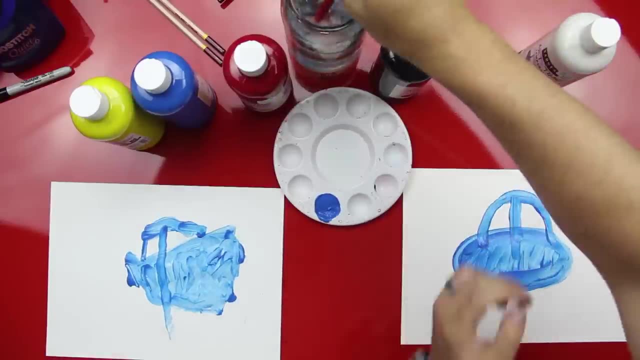 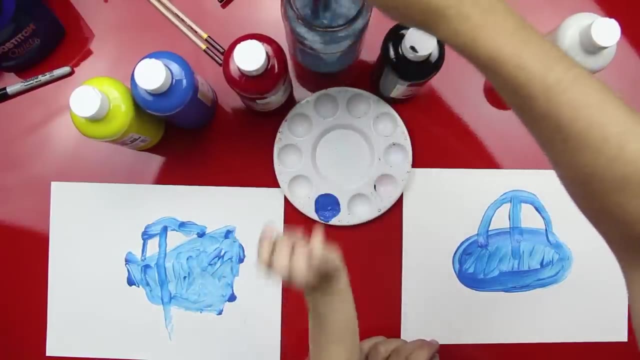 Cool, All right, take it easy. Okay, door. well, you can stop. all right, let's, let's, let's. wash off the blue. okay, we're done with blue and we're gonna switch to black. no, which one's black? you're right, that one's black. good job, yeah, that one's white. okay, we're almost done, we're. 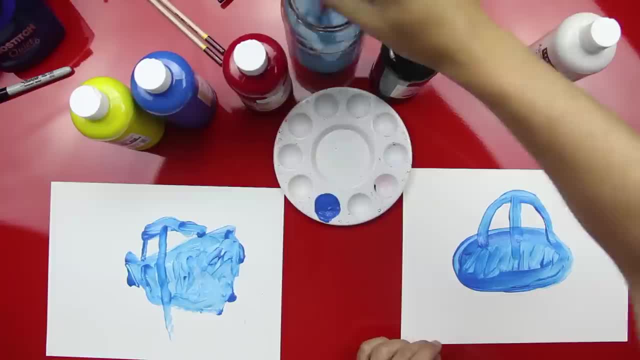 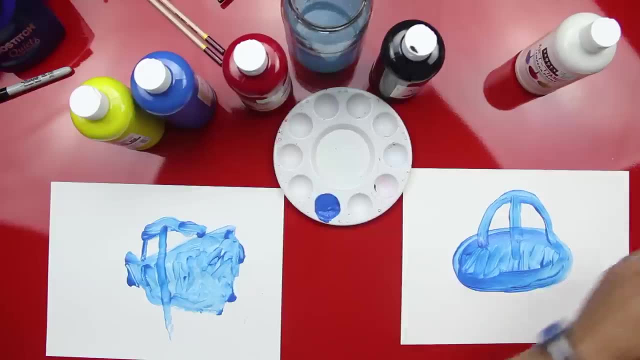 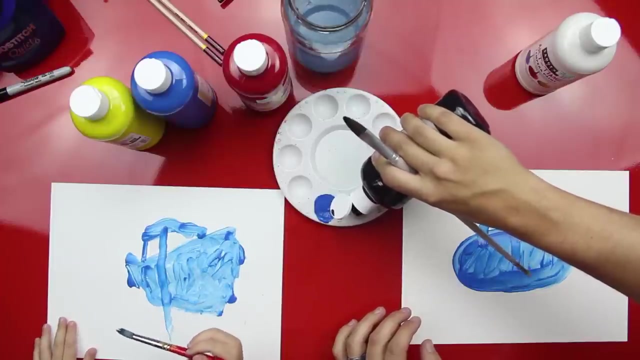 just gonna do the wheels you ready, all right. well, we could actually do. we could do some other things. we'll do some other things. here's your paper. you know, want to switch, ok, alright. okay, now we're going to use a black. yes, you tricked me. alright, get some black on your paint. 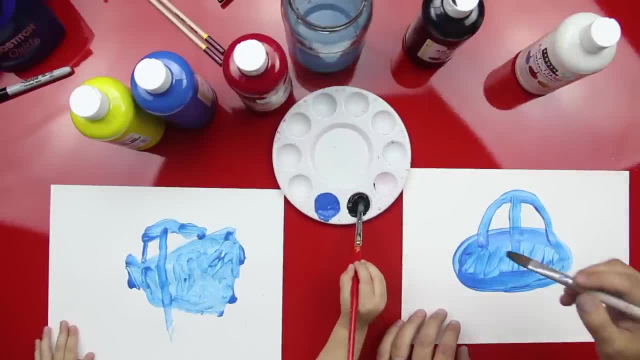 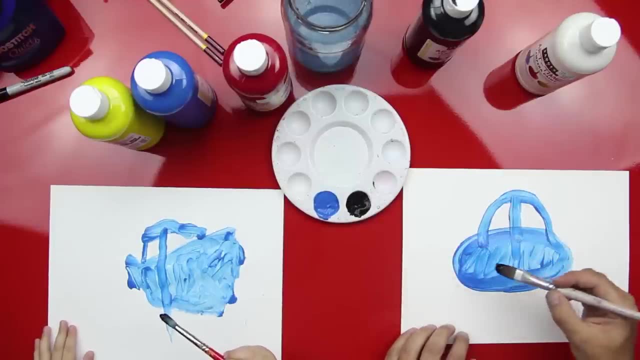 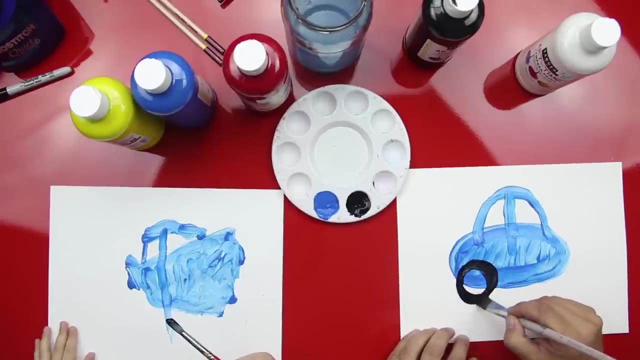 brush. hey, all right, good job. okay, watch dad, we're gonna do a wheel. you watch dad. okay, watch that, here we go, you're gonna do a wheel. okay, watch dad, here we go, we're gonna do a wheel, We can do that up. do a wheel, Do a round circle. Can you do a round circle? Yeah, Do a round circle, right. 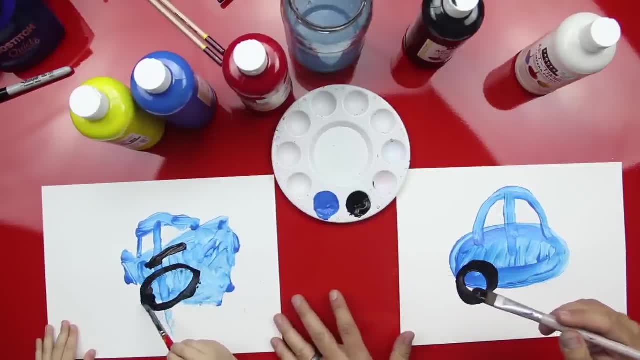 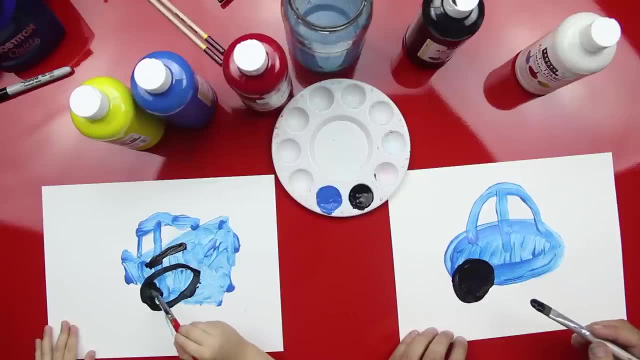 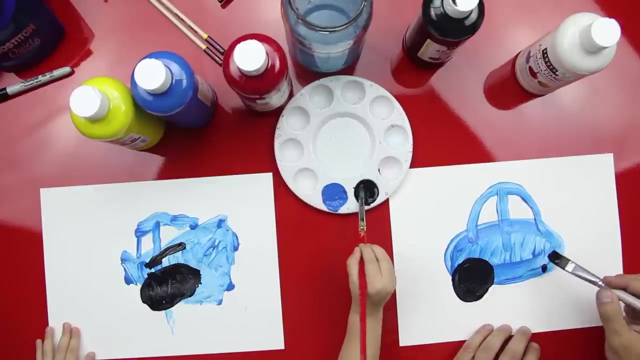 here. Yes, good job. Okay now, color in your circle, Color in your wheel. Can you paint it in? Did you burp? Yeah, You just got to say: excuse me, Excuse me, All right, get more black. Okay, we're going to do two wheels. You ready? Yeah, Watch that, Go as big circle. 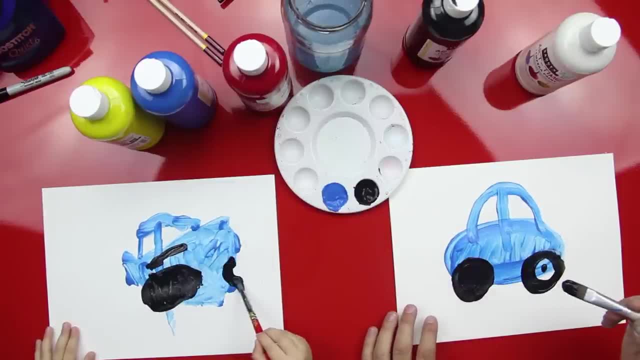 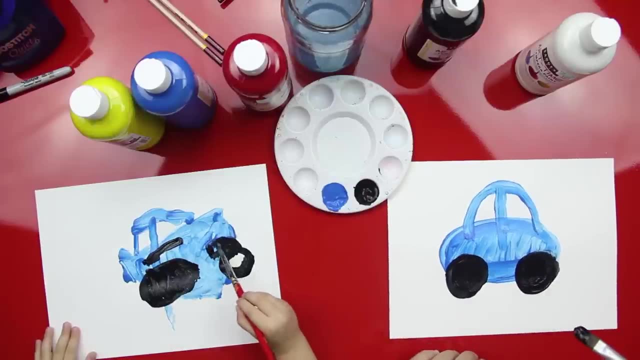 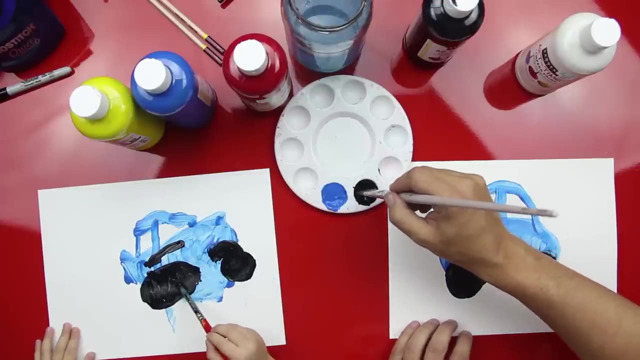 Can you do that? Do a big circle right here. Good job, Okay. now paint your circle in. Can you color it in? Yeah, Good job, Okay, all right, now we're going to paint the windows. Watch this, Austin. 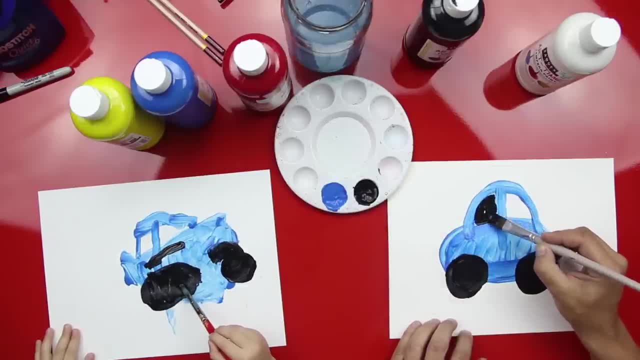 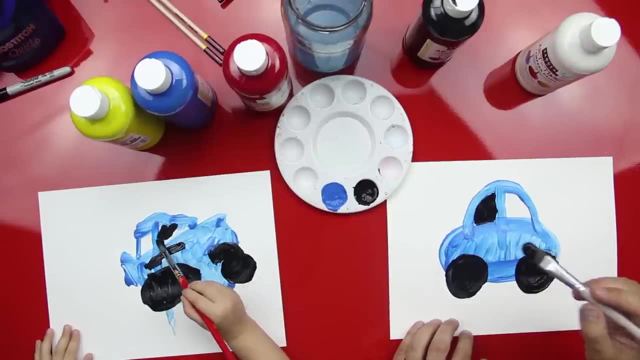 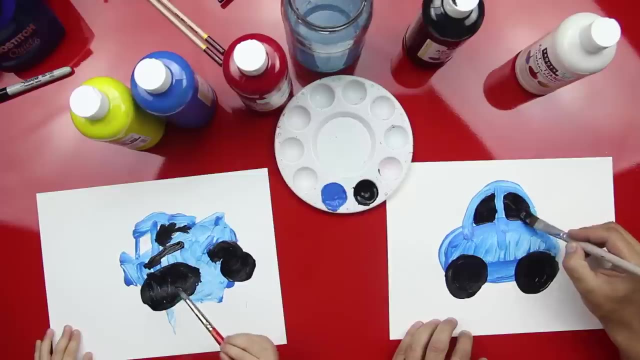 Austin, watch this. Paint inside the window. Can you paint in the window? Yep, just the white. Good job, Oops, I dripped. Okay, can you paint the other window? It dripped. Yeah, see, I got a little bit right there. 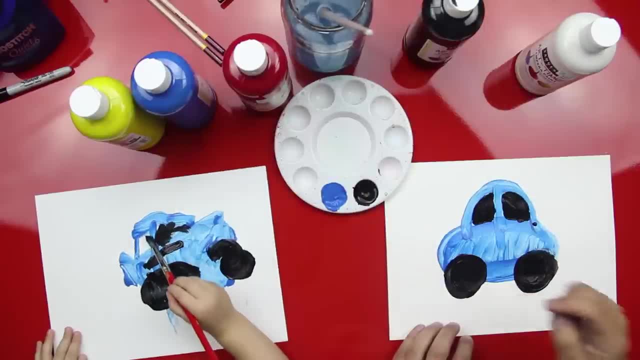 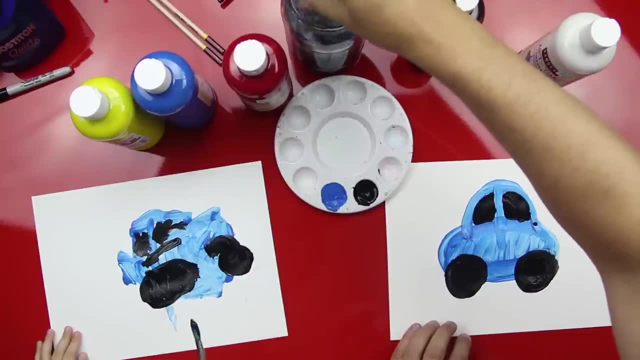 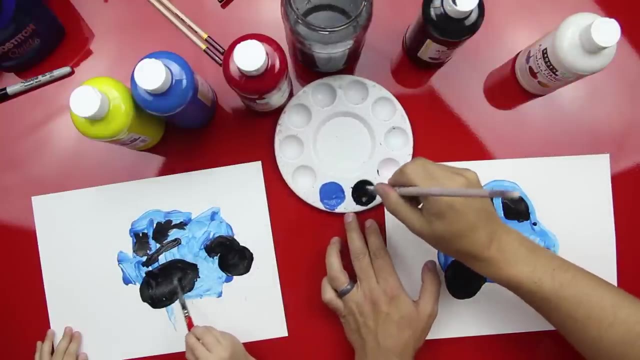 That's okay. Can you paint your window in? Paint this window. It's a flying car. It's a flying car. We need to paint the road. huh, Yeah, Should we paint the road first? Yeah, Okay, get a little more black, so it's not flying. Here we go, Get. 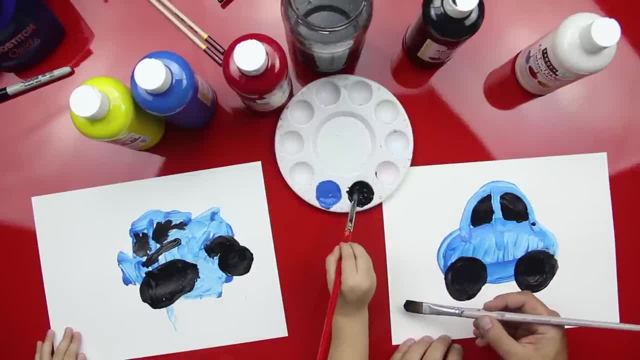 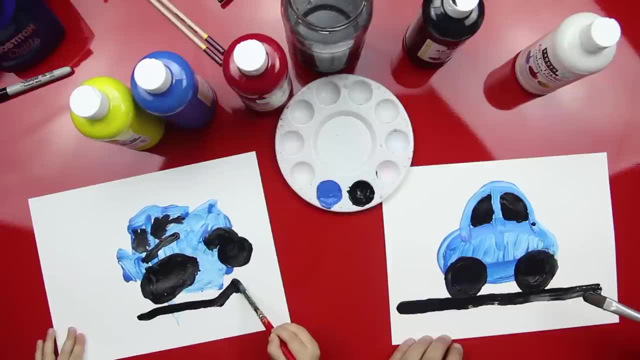 some more black. Watch this, Austin. Okay, let's paint the road. We're going to do a line that goes through right where the wheels are. Can you do that? It was still kind of fine, Good job, All right. oh, it's a round road, I like it. Okay, let's wash the black. 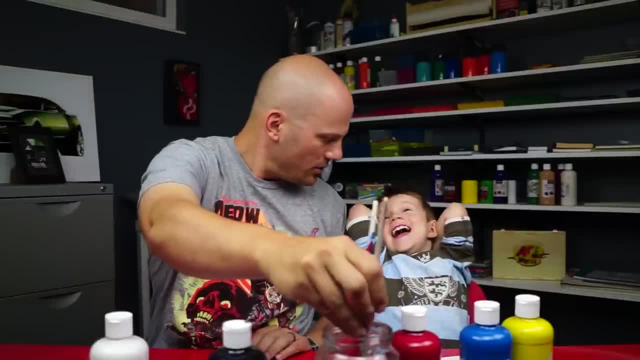 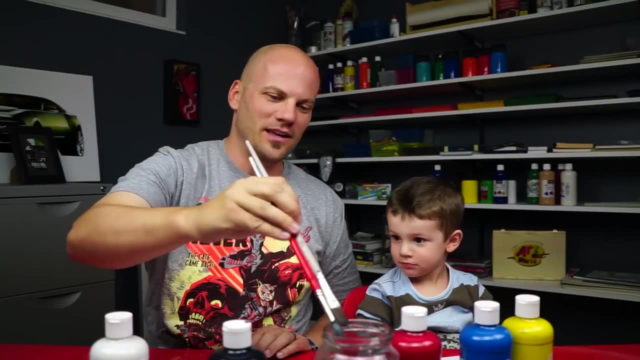 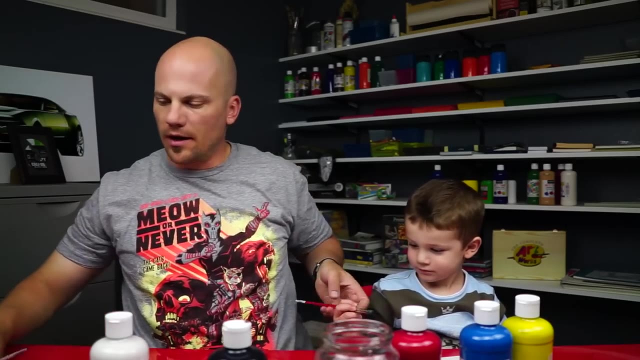 off. okay, Why. And then we're going to get white. Yeah, You ready for some white? Yeah, Okay, It's not working, It is working. Watch, I'll show you. You want the red paintbrush again? Yeah, Okay, here you go. All right, okay, now we're going to get some white and 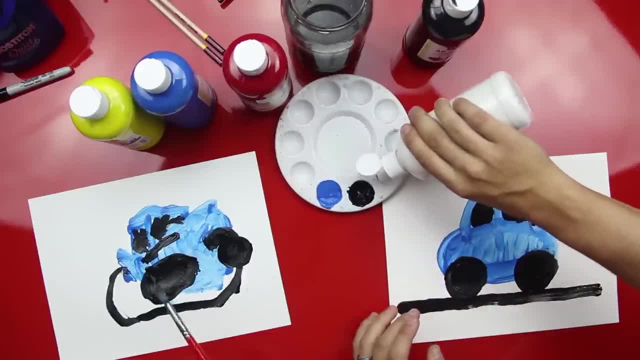 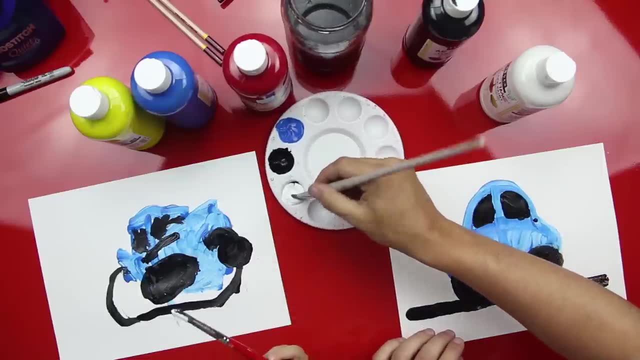 we're going to use the white for the wheels. We're going to finish the wheels. okay, Let's get a little white on your paintbrush. We got some black in there. huh, White, White. Okay, watch this. We're just going to do a dot inside. 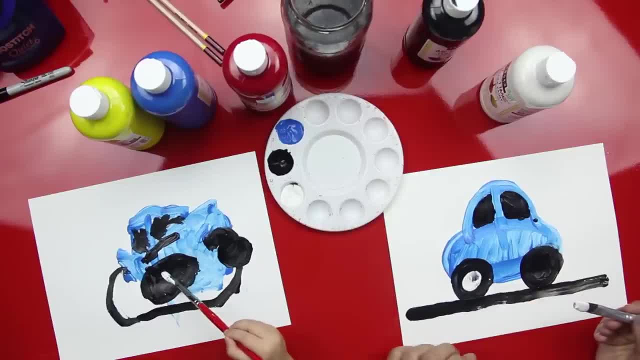 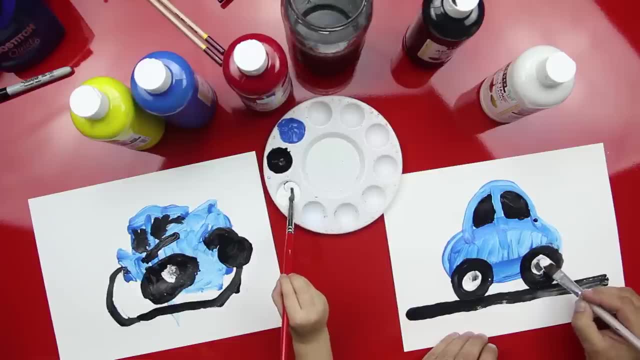 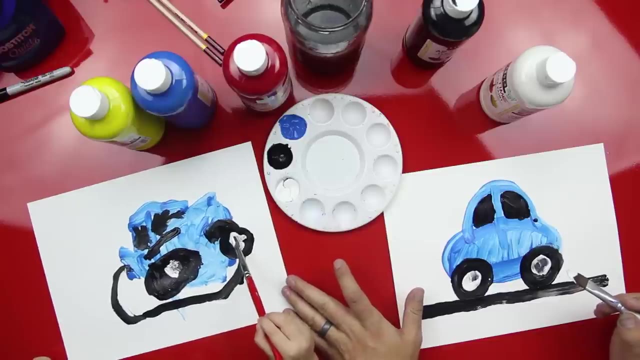 the wheel. Can you do a dot inside the wheel? Yeah, Yes, Okay, get some more white and we're going to do another dot inside this wheel. You see that. Yeah, Do this wheel. Yes, good job. That's the inside of the wheel. 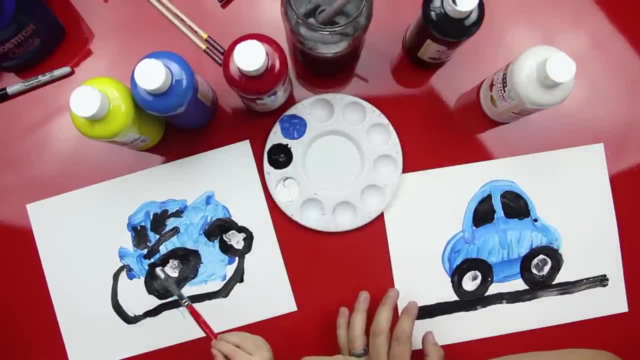 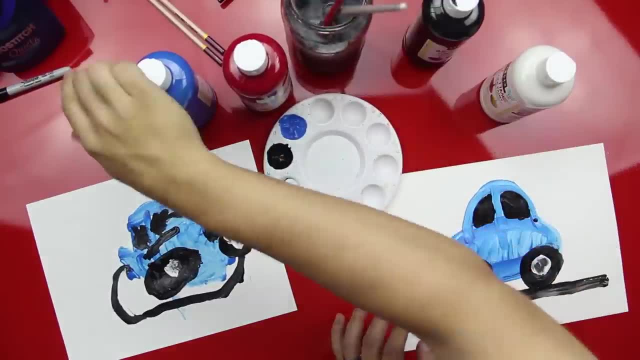 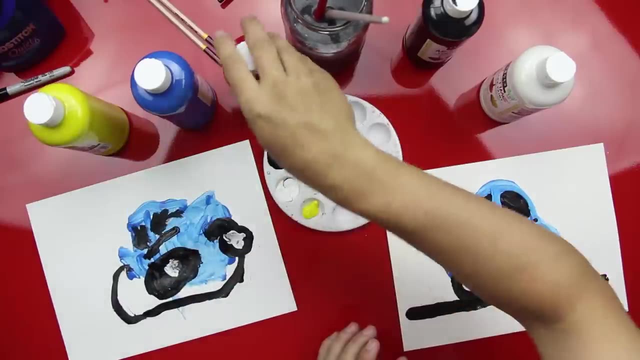 Is that cool? Okay, let's rinse off the white and we're going to do one last thing. We're going to get some yellow, Yellow, Yes, We're going to get some yellow, just a little bit, We don't need too much- And we're going to get some red. Okay, What's this for, Do you? 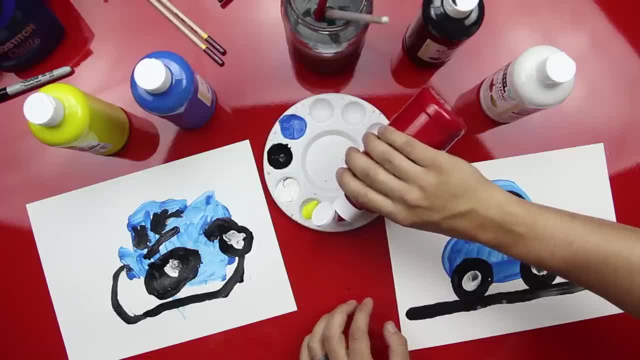 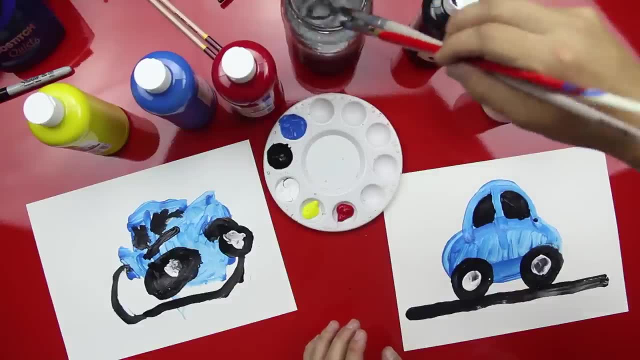 know what? this is going to be for Red. This is going to be for the lights- Lights. Okay, the lights on the front are going to be yellow And the lights on the back are going to be the red. They're going to be red, Okay, you. 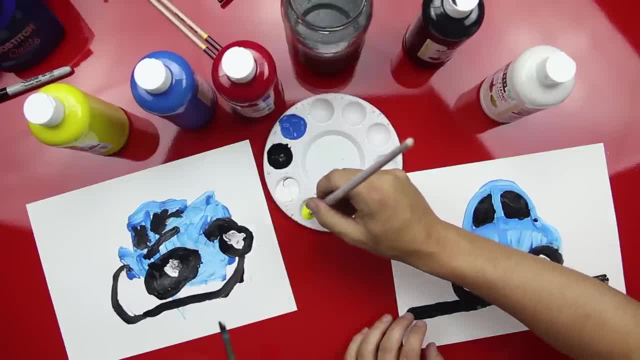 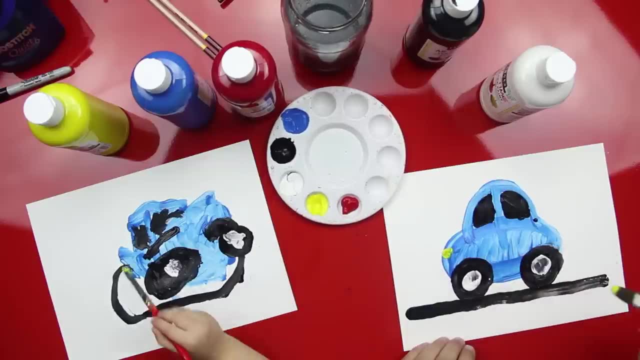 ready. Here's your paintbrush. We're almost done, You ready? Yeah, We're going to get some. what yellow, Yellow, Yellow? And then put a dot on the front car right there. Good job, Okay, rinse it off, I'll let you do it. Whoop, Wait, we're going to put red on the.